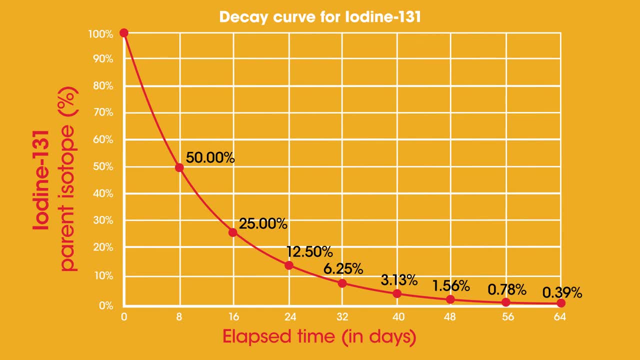 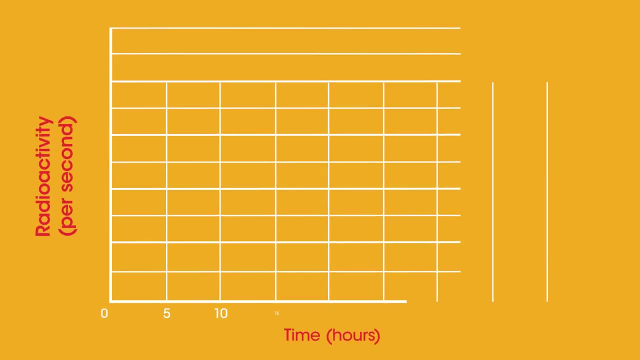 a graph like this. The graph is for the isotope iodine-131.. Notice how the count rate halves every eight days. So we say it has a half-life of eight days. Can you work out the half-life of the isotope? 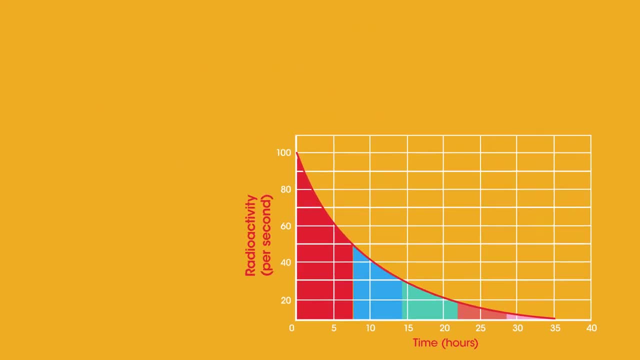 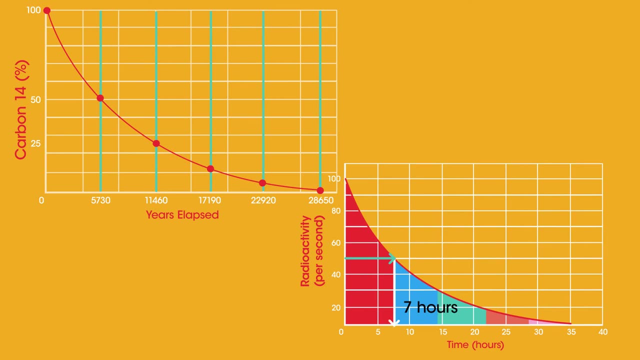 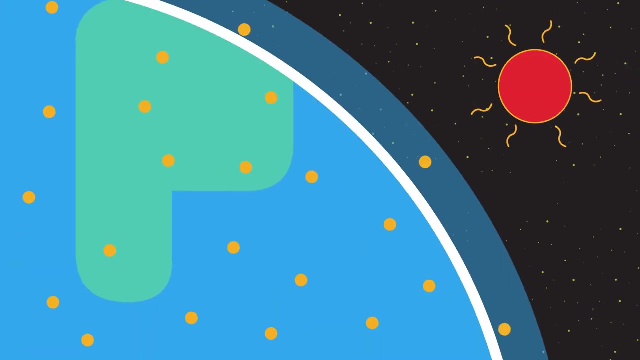 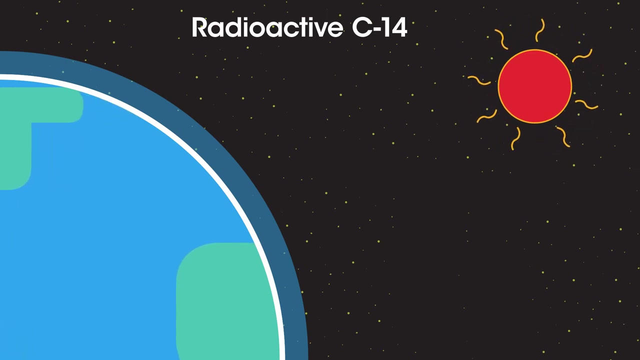 Let's remember this radioactive isotope. This is the decay curve for Carbon-14,, which all living things contain. It has a half-life of 5730 years. Atmospheric carbon dioxide contains a small but constant percentage of radioactive C14, made by the action of cosmic rays on nitrogen molecules. This enters all. 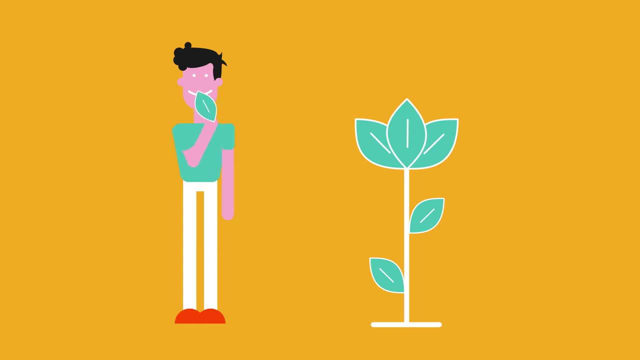 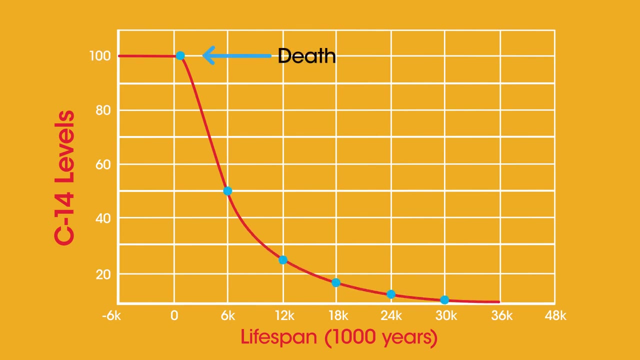 living organisms via photosynthesis and subsequent food chains, While living levels are constantly topped up, but upon death the amount decays away. The ratio of C14 to C12 gives us a way of estimating how many half-lives have passed since death. 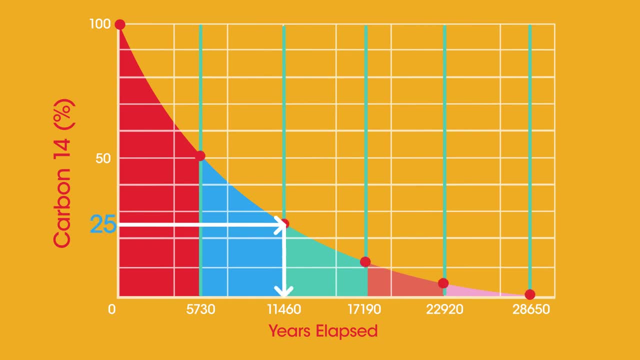 For example, if a lump of wood contains only 25% of the original content of C14,, then the wood has been dead for two half-lives, or 11,460 years. There is a limit to how far radiocarbon dating is reliable. 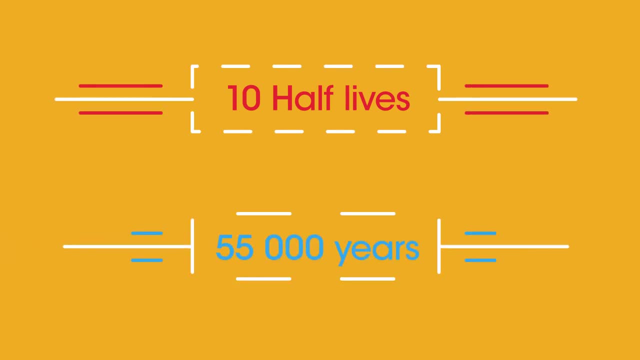 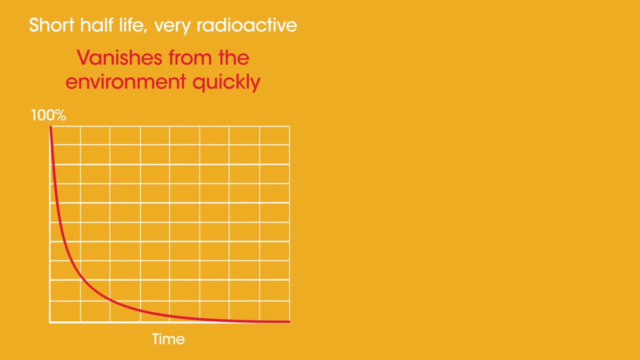 After about 10 half-lives or 55,000 years, there is so little C14 remaining that measuring it with any degree of accuracy is impossible. Short half-life radionuclides are used in medicine, So the patient is safe to go home in a few hours after dosage, whereas nuclear waste. 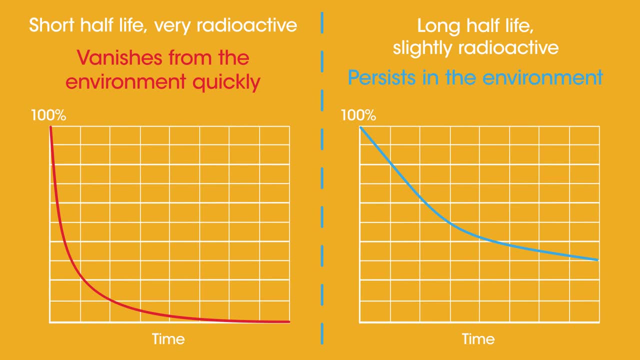 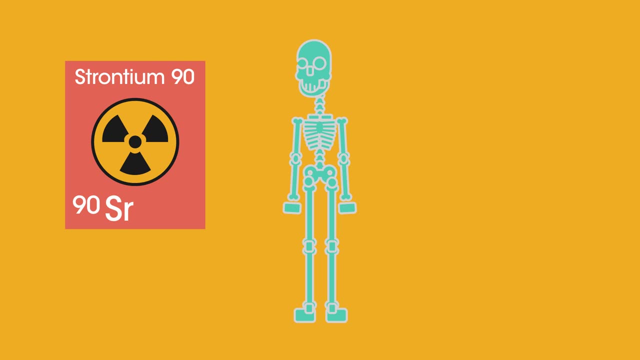 has a half-life of many tens of thousands of years. Most of the world's population have some strontium-90 in their skeleton, which originates from the atmospheric detonation of atomic weapons, mainly in the 1950s and 1960s.